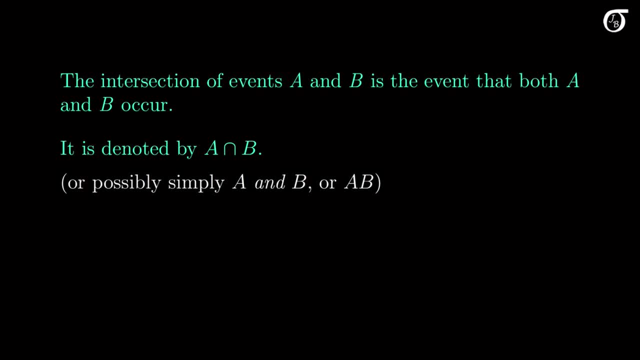 But you might also see A and B or possibly just AB representing the intersection. We are free to switch the ordering of the intersection of events. B intersect A, B and A is the same event as A intersect B, A and B. 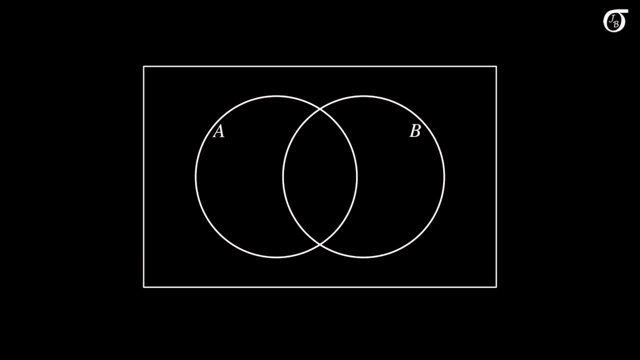 Here's a Venn diagram representation. The rectangle represents the sample space, the circle on the left represents event A and the circle on the right represents event B. The intersection of A and B is this green region, which is in both A and B. 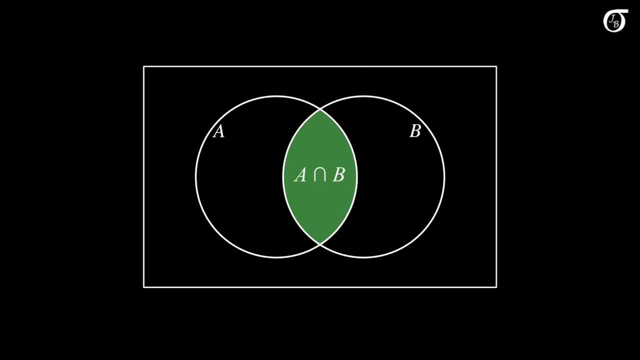 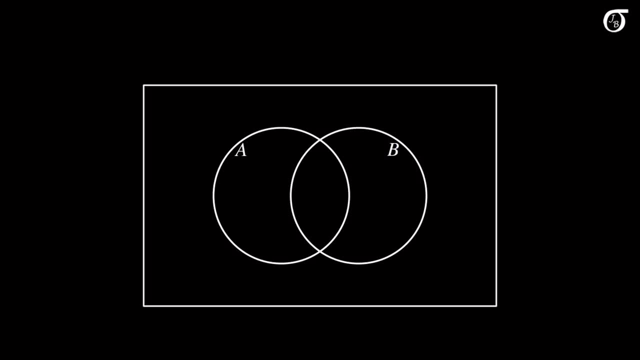 It is where both A and B occur. Here's another visual representation of events A and B. Now let's suppose we start pushing the circles apart A little further. a little further, there we go. Let's look at this scenario where A and B do not overlap. 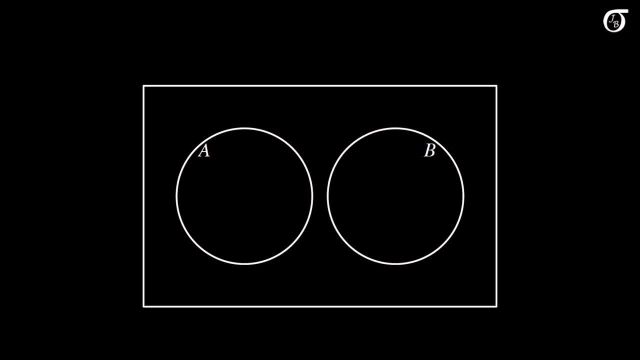 Here A and B do not share any common ground. They share no part of the sample space and they cannot both occur. We might casually say that they don't have an intersection, but mathematicians prefer to say that their intersection is the empty set. 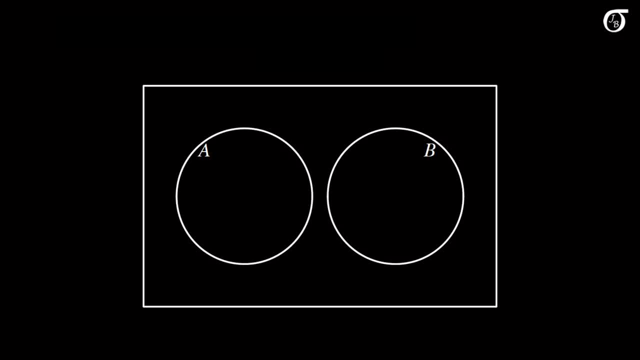 Their intersection contains no elements. In this situation we say that A and B are mutually exclusive. The intersection of mutually exclusive events contains no sample points, so the probability of their intersection is zero. Mutually exclusive events are sometimes called disjoint events. The union of events A and B is the intersection of A and B. 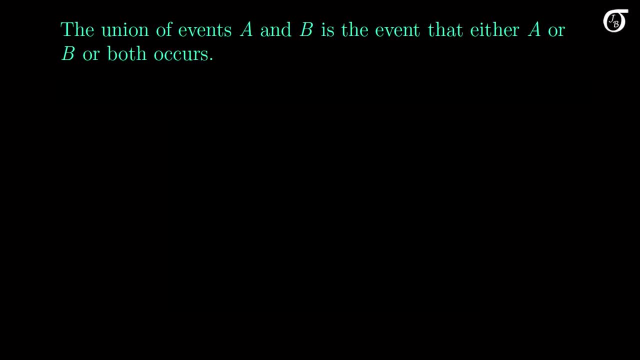 This is the event that either A or B or both occurs In set notation. the union is denoted by this union symbol: A, union B, But you might simply see A or B. When we use the term A or B in probability we are referring to their union. 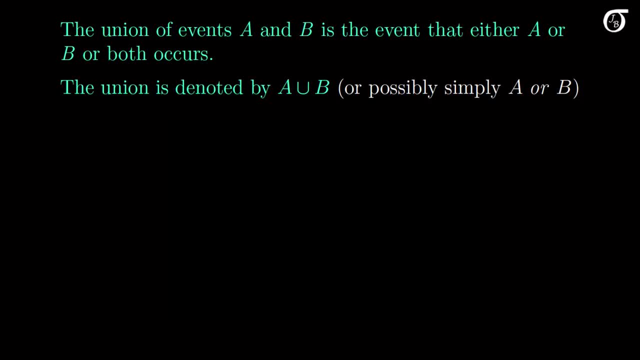 and using the word or in the inclusive sense, A or B means A or B or both. We are also free to switch the ordering in the union of events. A union A, B or A is the same event as A union B, A or B. 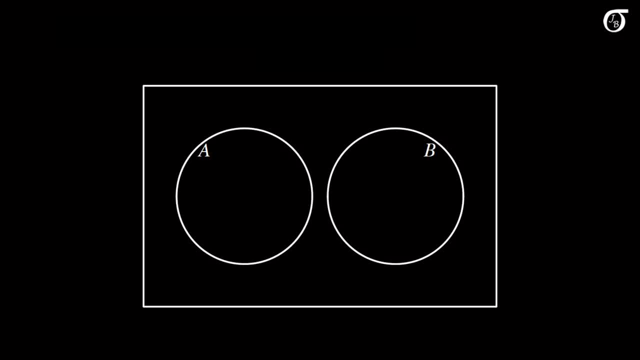 Their intersection contains no elements. In this situation we say that A and B are mutually exclusive. The intersection of mutually exclusive events contains no sample points, so the probability of their intersection is zero. Mutually exclusive events are sometimes called disjoint events. The union of events A and B is the intersection of A and B. 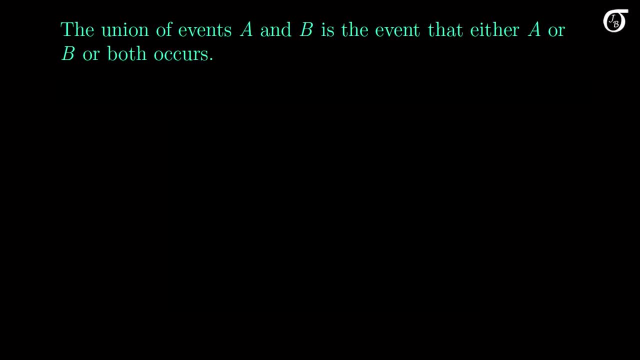 This is the event that either A or B or both occurs In set notation. the union is denoted by this union symbol: A, union B, But you might simply see A or B. When we use the term A or B in probability we are referring to their union. 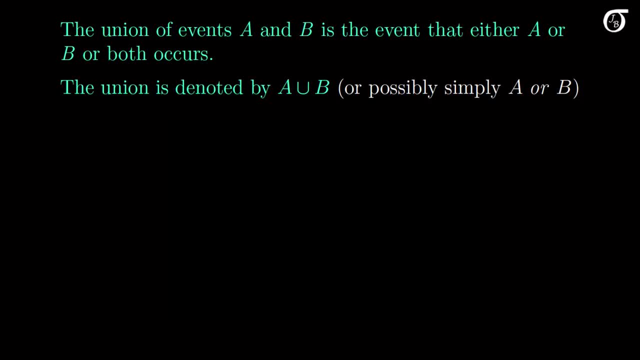 and using the word or in the inclusive sense, A or B means A or B or both. We are also free to switch the ordering in the union of events. A union A, B or A is the same event as A union B, A or B. 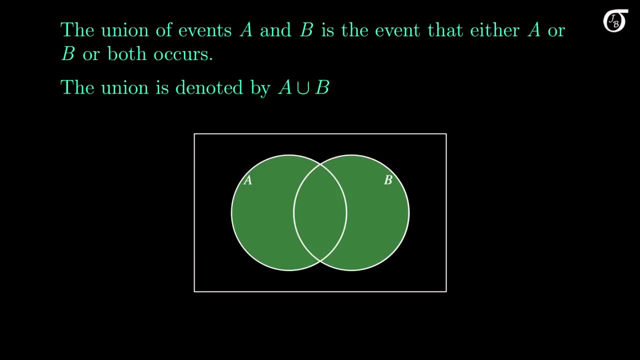 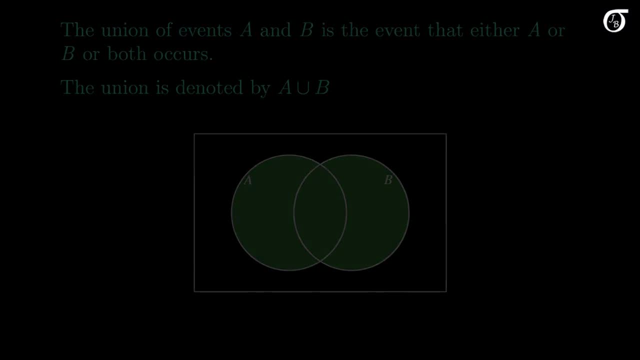 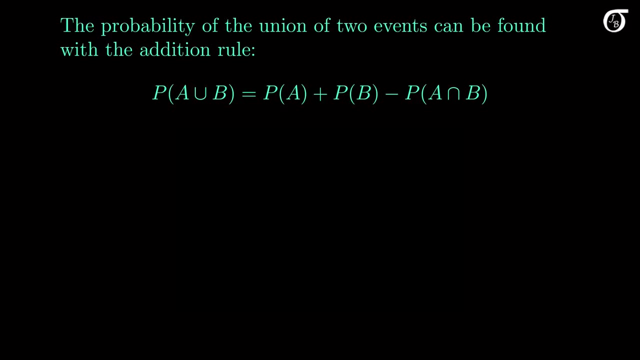 Here's a Venn diagram: representation of events A and B. The green region represents the union, everything that is in either A or B or both. The probability of the union of two events can be found with the addition rule. The probability of the union of A and B is the sum of the individual probabilities. 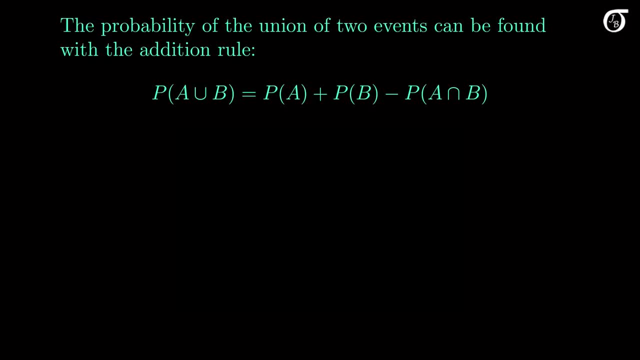 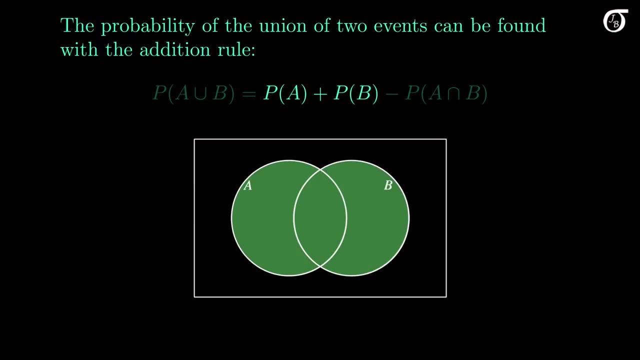 minus the probability of the intersection. Why is that? Well, let's take a look at the Venn diagram. If we add the probability of A to the probability of B, then we've added the probability of this intersection twice, because the intersection occurs in both A and B. 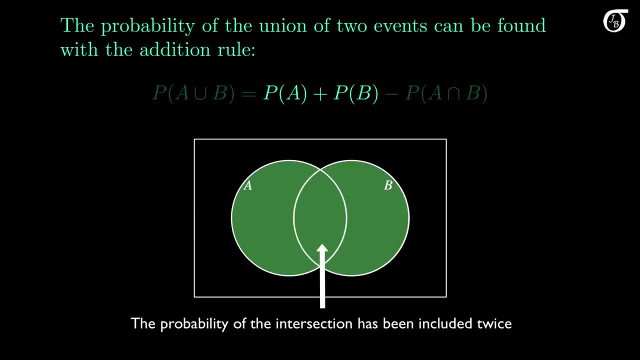 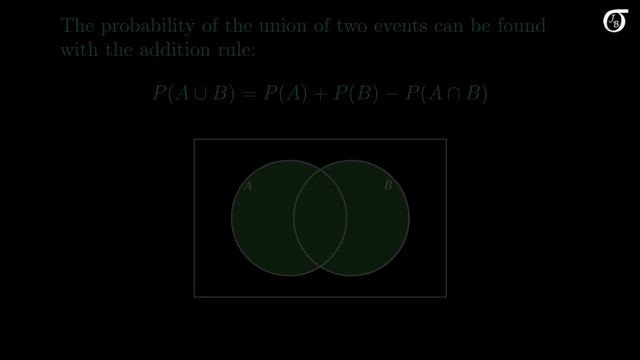 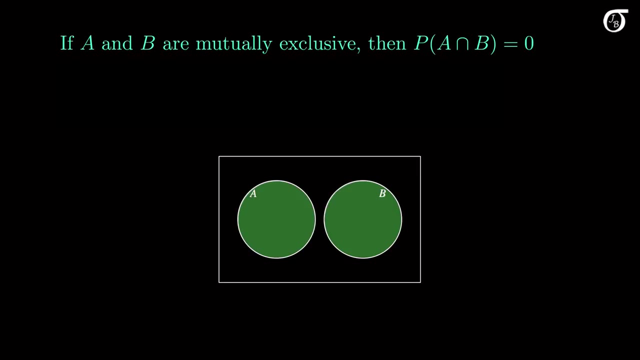 The probability of the intersection should only be included once. so we need to subtract one of those And that end result is called the addition rule. Recall that if A and B are mutually exclusive, then they don't share any sample points, they don't share any common ground. 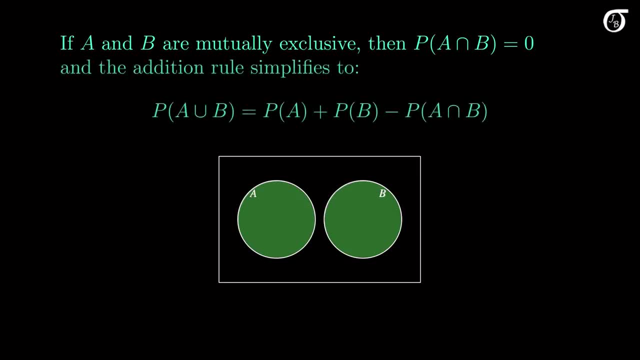 and the probability of their intersection is zero. So if A and B are mutually exclusive events, then the addition rule simplifies to this where the probability of the union is equal to the sum of the individual probabilities. This is sometimes referred to as the special addition rule. 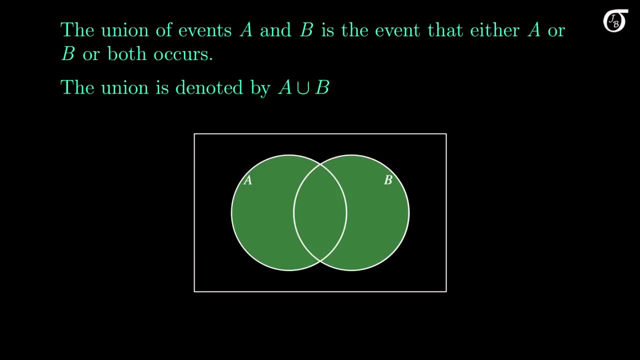 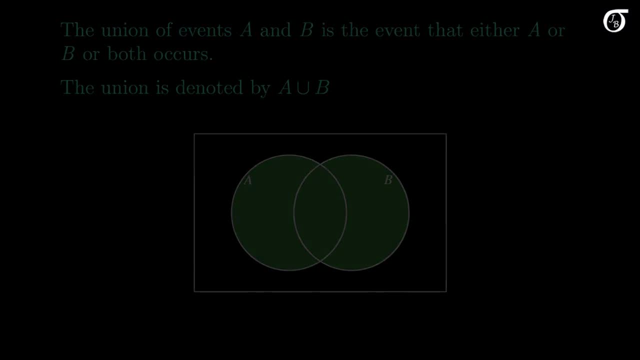 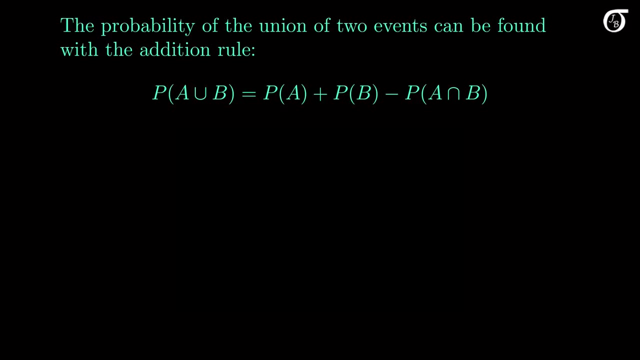 Here's a Venn diagram: representation of events A and B. The green region represents the union, everything that is in either A or B or both. The probability of the union of two events can be found with the addition rule. The probability of the union of A and B is the sum of the individual probabilities. 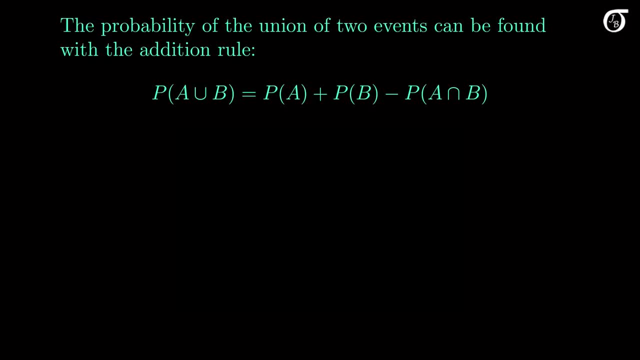 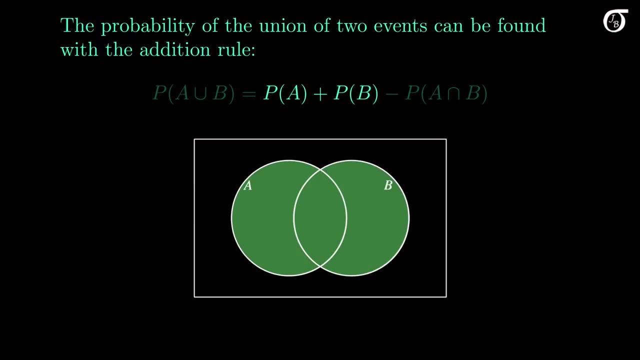 minus the probability of the intersection. Why is that? Well, let's take a look at the Venn diagram. If we add the probability of A to the probability of B, then we've added the probability of this intersection twice, because the intersection occurs in both A and B. 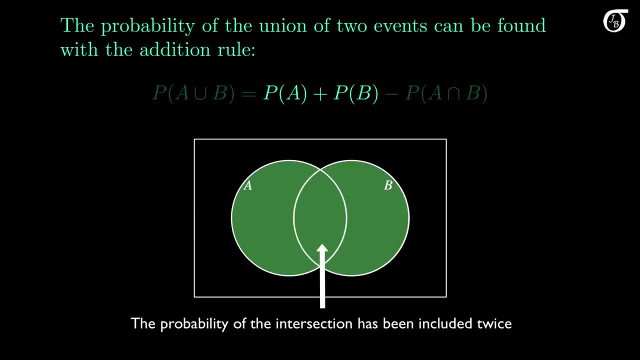 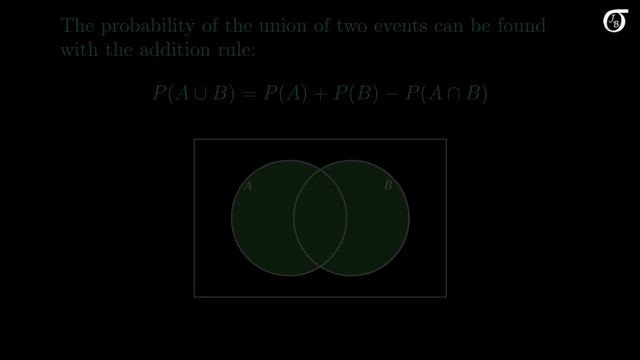 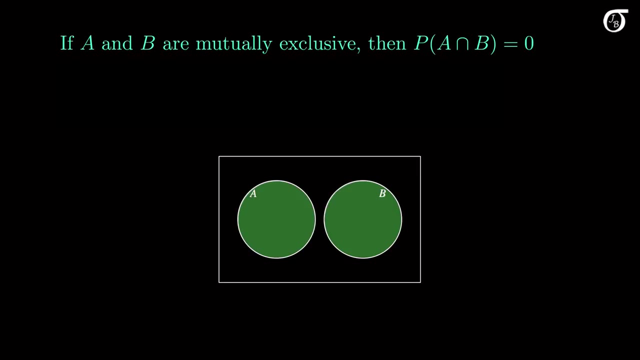 The probability of the intersection should only be included once. so we need to subtract one of those And that end result is called the addition rule. Recall that if A and B are mutually exclusive, then they don't share any sample points, they don't share any common ground. 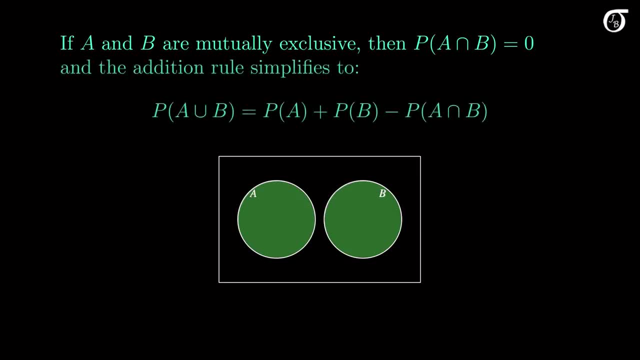 and the probability of their intersection is zero. So if A and B are mutually exclusive events, then the addition rule simplifies to this where the probability of the union is equal to the sum of the individual probabilities. This is sometimes referred to as the special addition rule. 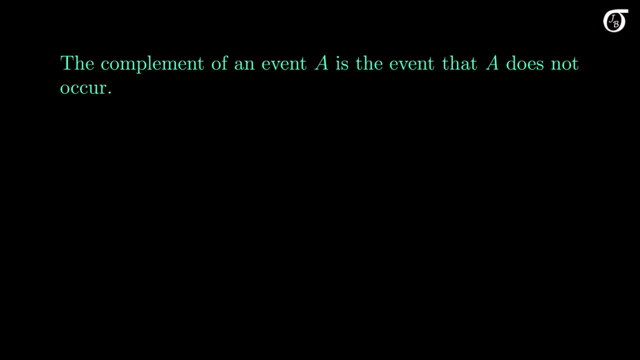 The complement of an event. A is the event that A does not occur. A little more formally, A complement is the set of all sample points in the sample space that are not in A. The complement of event A is often denoted by A bar. 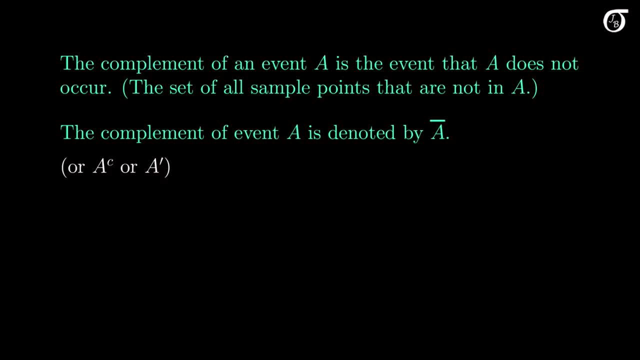 but you may also see A with a superscript, C or A prime. All three of these are very commonly used to denote the complement, so it's not a bad idea to get comfortable with all of them. Here's a Venn diagram representation of the sample space. 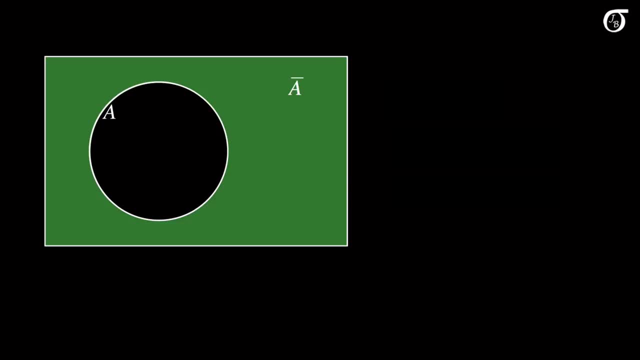 The black circle represents event A and the green region represents A complement. A complement is everything in the sample space that is not in A. A and A complement are mutually exclusive events and together they make up the entire sample space. Take note of three things. 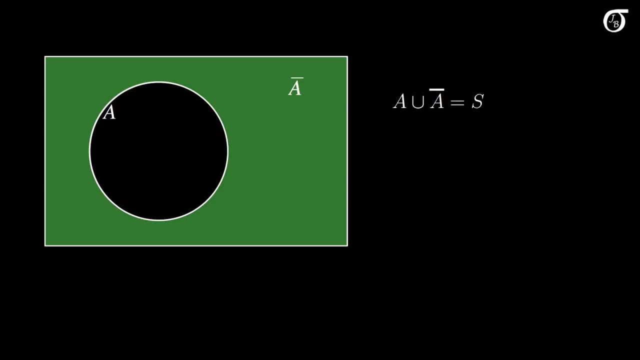 The union of A and A complement is the entire sample space And since A and A complement are mutually exclusive and the probability of the sample space is 1,, this implies that the sum of the probabilities of A and A complement is 1.. 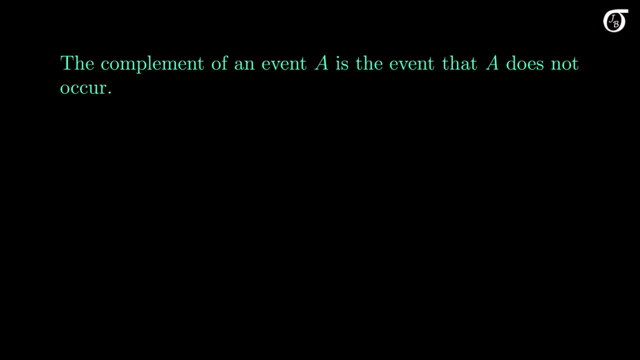 The complement of an event. A is the event that A does not occur. A little more formally, A complement is the set of all sample points in the sample space that are not in A. The complement of event A is often denoted by A bar. 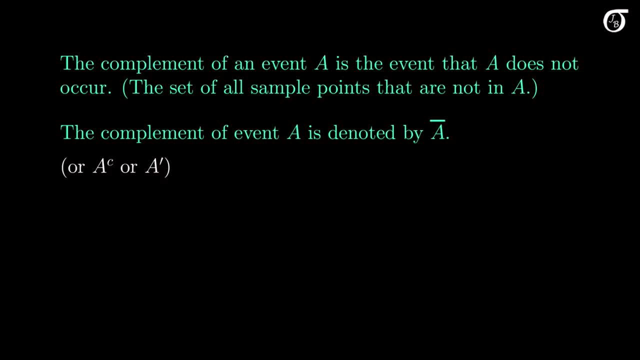 but you may also see A with a superscript, C or A prime. All three of these are very commonly used to denote the complement, so it's not a bad idea to get comfortable with all of them. Here's a Venn diagram representation of the sample space. 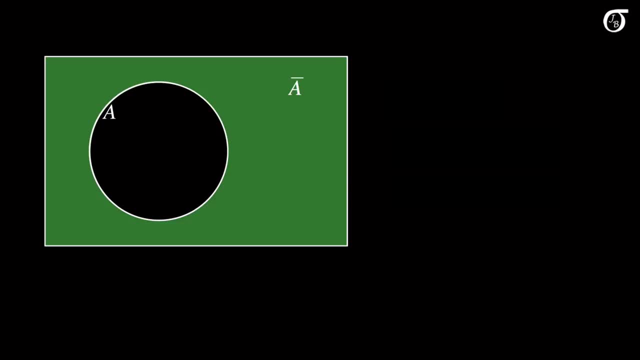 The black circle represents event A and the green region represents A complement. A complement is everything in the sample space that is not in A. A and A complement are mutually exclusive events and together they make up the entire sample space. Take note of three things. 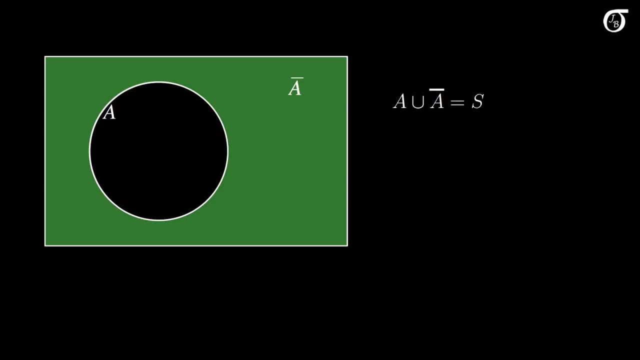 The union of A and A complement is the entire sample space And since A and A complement are mutually exclusive and the probability of the sample space is 1,, this implies that the sum of the probabilities of A and A complement is 1.. 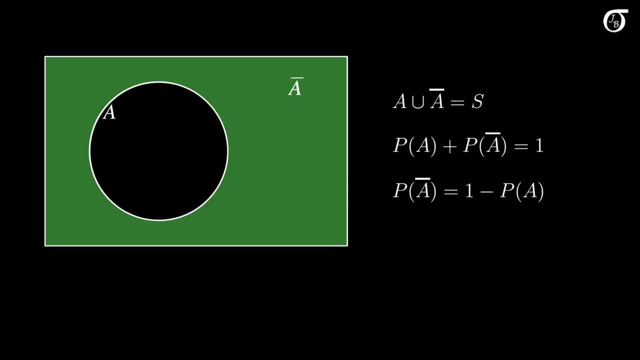 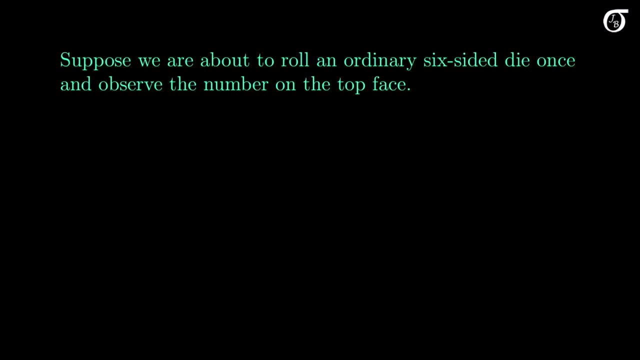 And finally, the probability of A complement is 1 minus the probability of A. We'll often use this complement rule in probability problems, although sometimes it's so natural that we won't even consciously realize we're using it. Let's work through a simple example to illustrate some of these concepts. 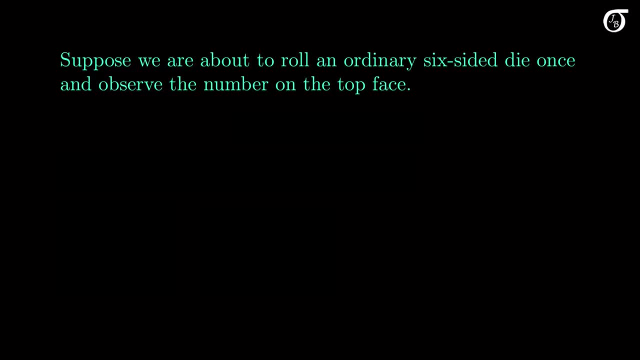 Suppose we are about to roll an ordinary 6-sided die once and observe the number on the top face. Here's a natural way to define the sample space, the set of the 6 possible outcomes, If it's an ordinary die and we're rolling it fairly. 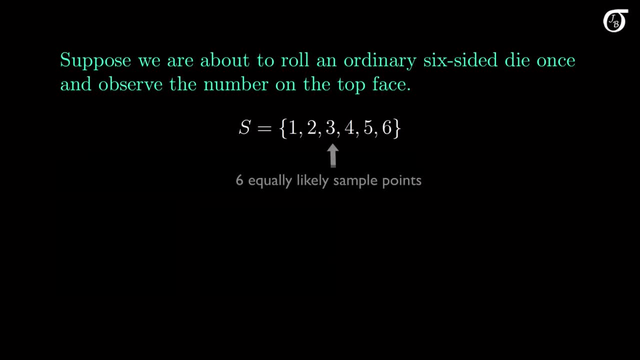 then it's reasonable to think that these 6 sample points are equally likely. That won't be perfectly true in practice, but it's a reasonable approximation to reality in this type of scenario. And suppose we define the following events: E is the odd numbers, F is the values greater than 3,. 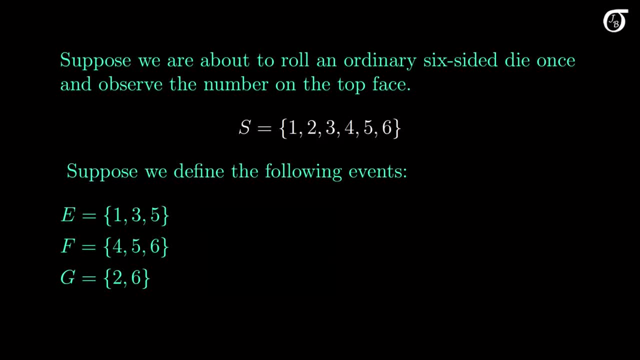 and G is made up of the numbers 2 and 6.. Since the outcomes are equally likely, we know that the probability of E is 3 over 6 or a half. the probability of F is also 3 over 6 or a half. 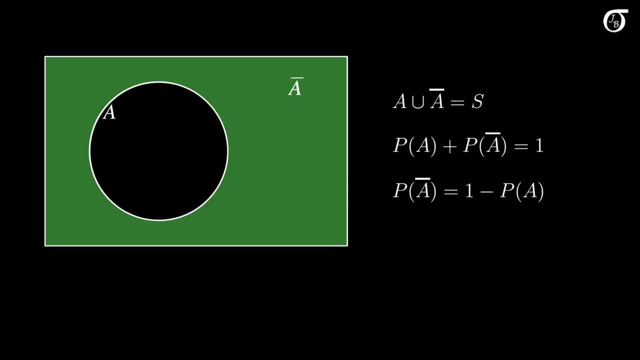 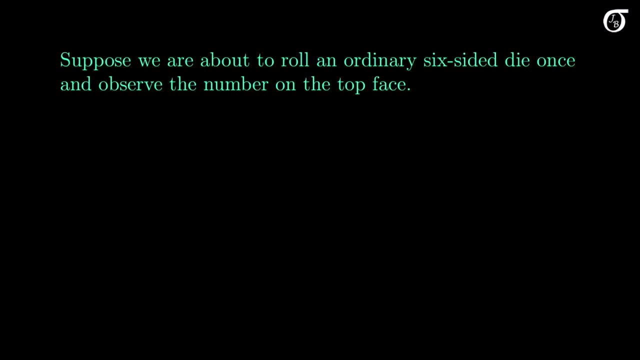 And finally, the probability of A complement is 1 minus the probability of A. We'll often use this complement rule in probability problems, although sometimes it's so natural that we won't even consciously realize we're using it. Let's work through a simple example to illustrate some of these concepts. 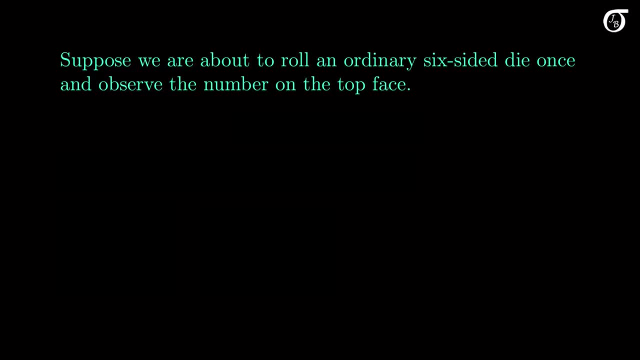 Suppose we are about to roll an ordinary 6-sided die once and observe the number on the top face. Here's a natural way to define the sample space, the set of the 6 possible outcomes, If it's an ordinary die and we're rolling it fairly. 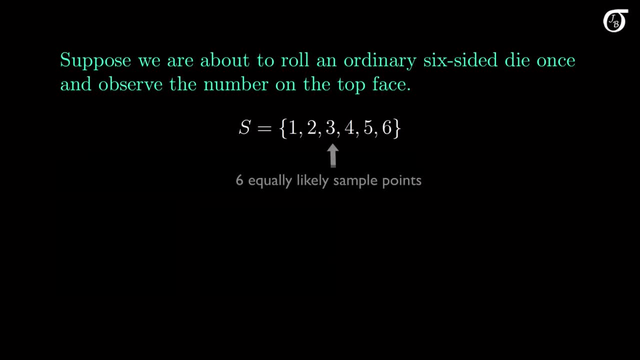 then it's reasonable to think that these 6 sample points are equally likely. That won't be perfectly true in practice, but it's a reasonable approximation to reality in this type of scenario. And suppose we define the following events: E is the odd numbers, F is the values greater than 3,. 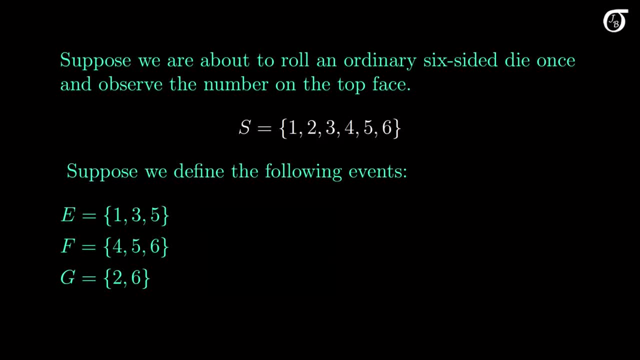 and G is made up of the numbers 2 and 6.. Since the outcomes are equally likely, we know that the probability of E is 3 over 6 or a half. the probability of F is also 3 over 6 or a half. 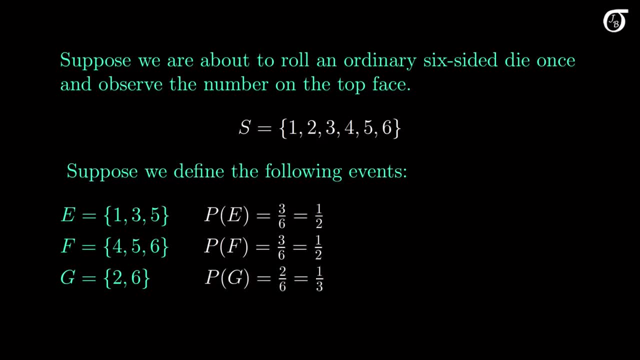 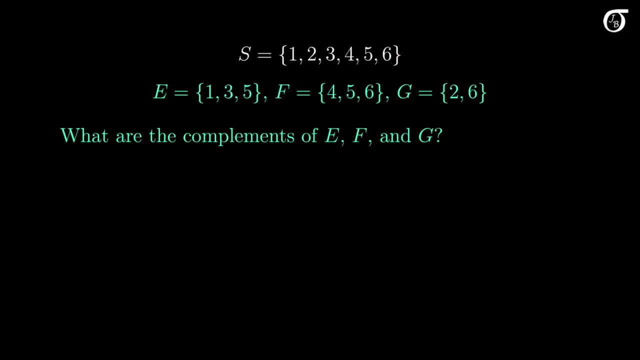 and the probability of G is 2 over 6 or a third. What are the complements of events E, F and G? E complement is made up of everything in the sample space that is not in E, so the event E complement is the even numbers 2,, 4, and 6.. 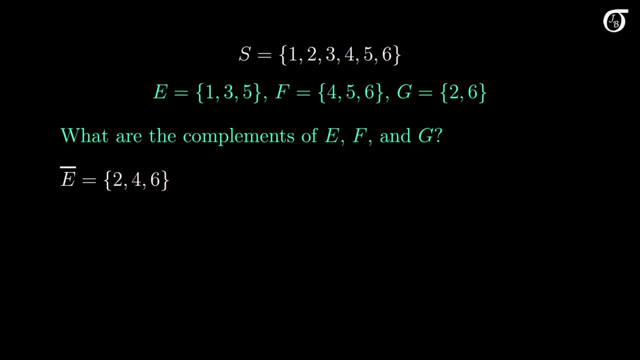 What is the probability of E complement? E complement is made up of 3 numbers- 2,, 4, and 6, and there are 6 equally likely possibilities in the sample space. so the probability of E complement is 3 over 6.. 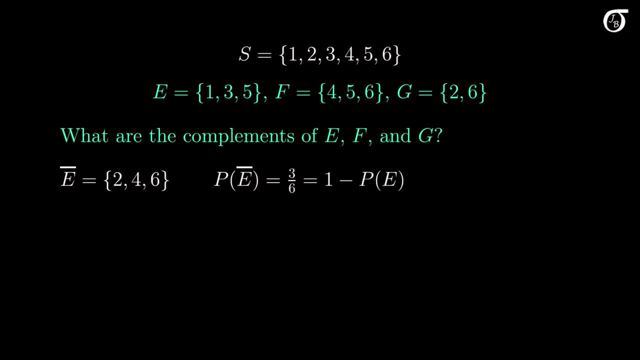 Note that this is equal to 1 minus the probability of event E. Event F is made up of the numbers that are greater than 3, so F complement is made up of the numbers that are less than or equal to 3, the sample points 1,, 2, and 3.. 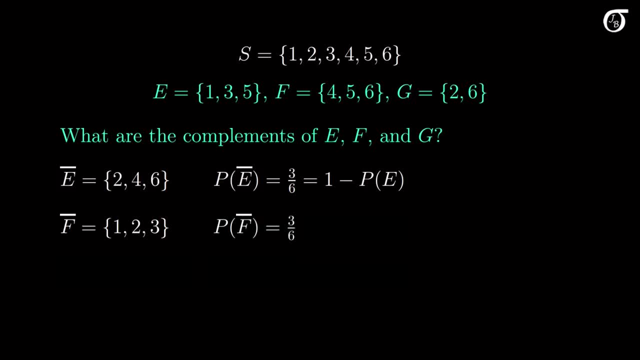 The probability of F complement is thus 3 over 6, and this also equals 1 minus the probability of F. G is made up of the numbers 2 and 6,, so G complement is made up of the other numbers in the sample space. 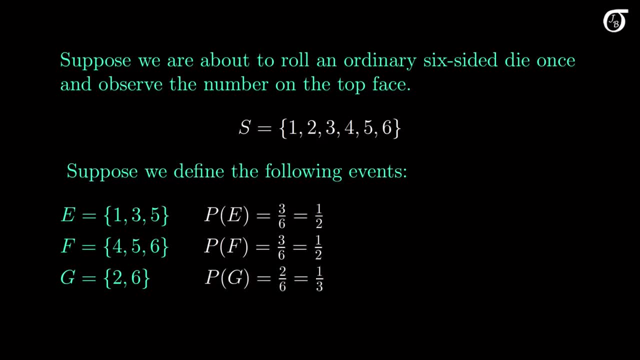 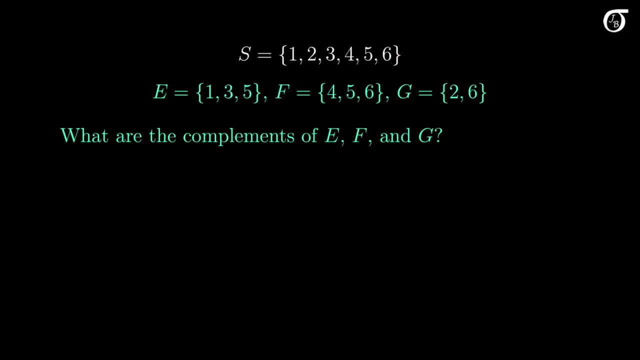 and the probability of G is 2 over 6 or a third. What are the complements of events E, F and G? E complement is made up of everything in the sample space that is not in E, so the event E complement is the even numbers 2,, 4, and 6.. 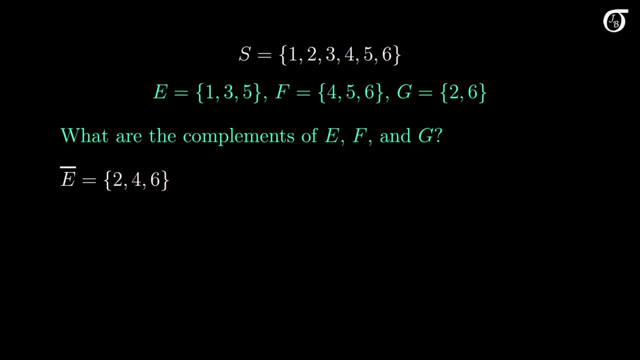 What is the probability of E complement? E complement is made up of 3 numbers- 2,, 4, and 6, and there are 6 equally likely possibilities in the sample space. so the probability of E complement is 3 over 6.. 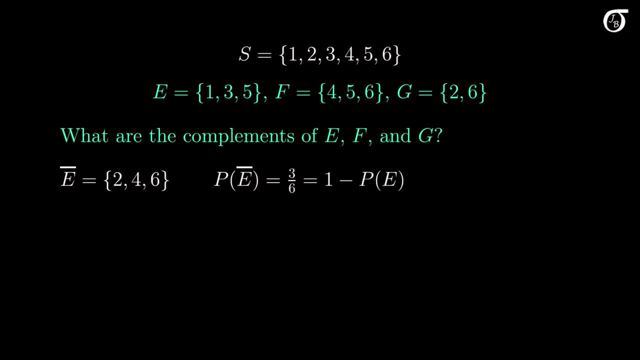 Note that this is equal to 1 minus the probability of event E. Event F is made up of the numbers that are greater than 3, so F complement is made up of the numbers that are less than or equal to 3, the sample points 1,, 2, and 3.. 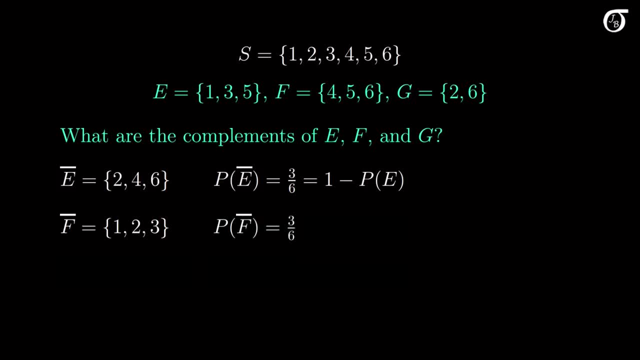 The probability of F complement is thus 3 over 6, and this also equals 1 minus the probability of F. G is made up of the numbers 2 and 6,, so G complement is made up of the other numbers in the sample space. 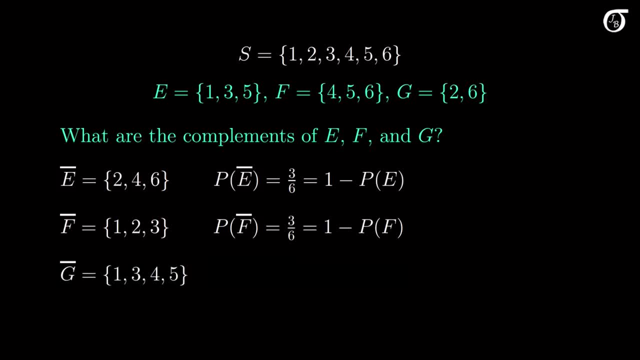 1,, 3,, 4, and 5.. The probability of G complement is thus 4 over 6, and of course this equals 1 minus the probability of G. Now suppose we're interested in the pairwise intersections. The intersection of E and F is the set of sample points that are in both E and F. 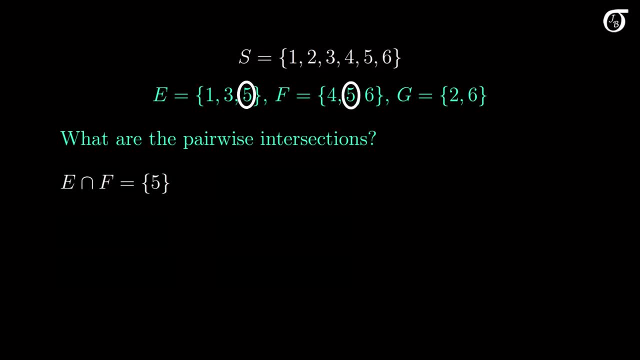 and here that's just the number 5, that's the only sample point in the sample space that occurs in both E and F. Since the intersection is made up of 1 out of the 6 equally likely outcomes, the probability of their intersection is 1 out of 6.. 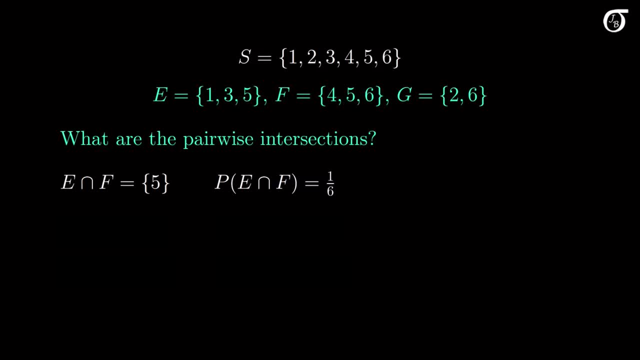 The intersection of E and G is the set of sample points that are in both E and G, but there are no elements of the sample space that occur in both. so the intersection between E and G is the empty set. We sometimes use this symbol to represent the empty set. 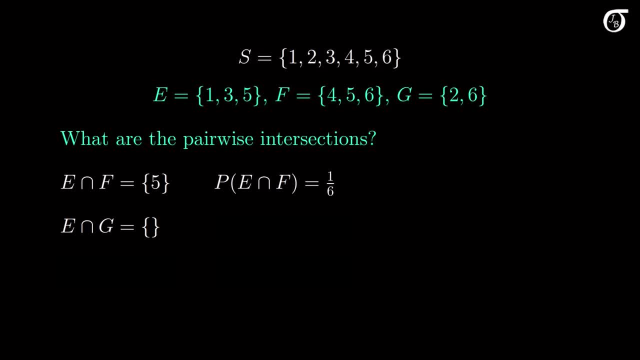 E and G are mutually exclusive. they cannot both occur on the same roll, and the probability of their intersection is 0.. The F and G intersection contains just the number 6, and the probability of that intersection is 1 out of 6.. 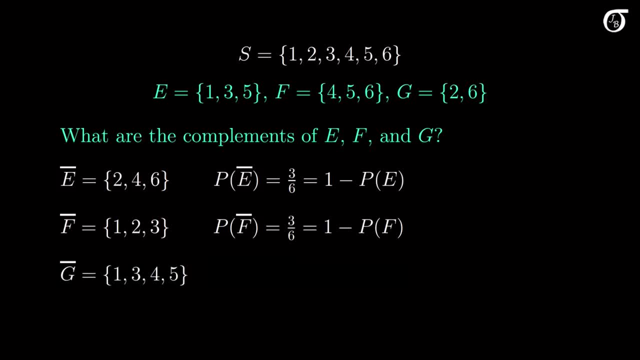 1,, 3,, 4, and 5.. The probability of G complement is thus 4 over 6, and of course this equals 1 minus the probability of G. Now suppose we're interested in the pairwise intersections. The intersection of E and F is the set of sample points that are in both E and F. 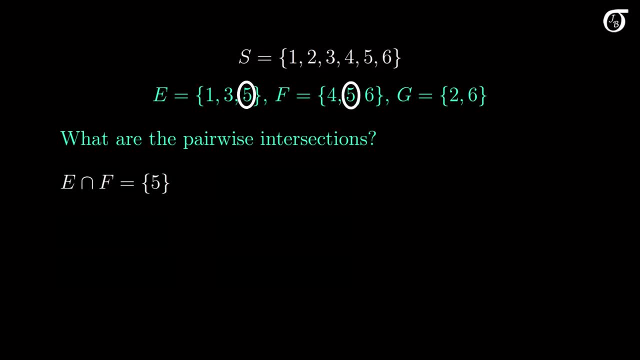 and here that's just the number 5, that's the only sample point in the sample space that occurs in both E and F. Since the intersection is made up of 1 out of the 6 equally likely outcomes, the probability of their intersection is 1 out of 6.. 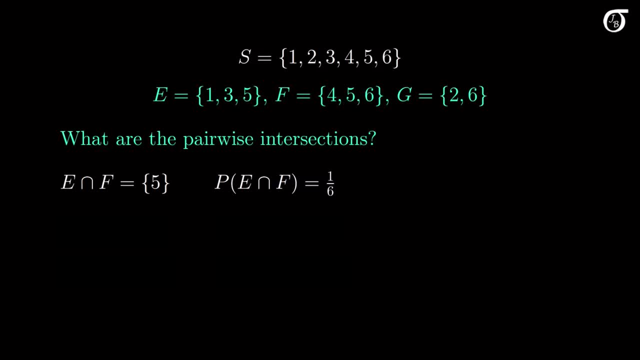 The intersection of E and G is the set of sample points that are in both E and G, but there are no elements of the sample space that occur in both. so the intersection between E and G is the empty set. We sometimes use this symbol to represent the empty set. 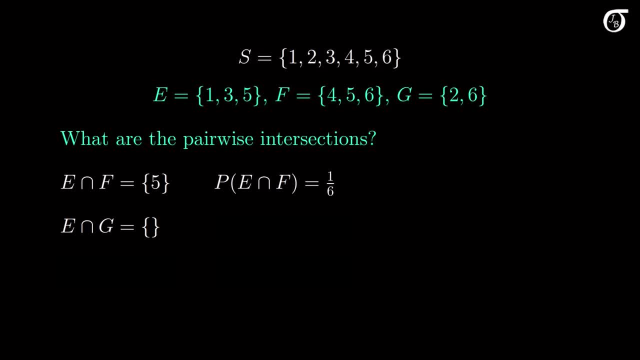 E and G are mutually exclusive. they cannot both occur on the same roll, and the probability of their intersection is 0.. The F and G intersection contains just the number 6, and the probability of that intersection is 1 out of 6.. 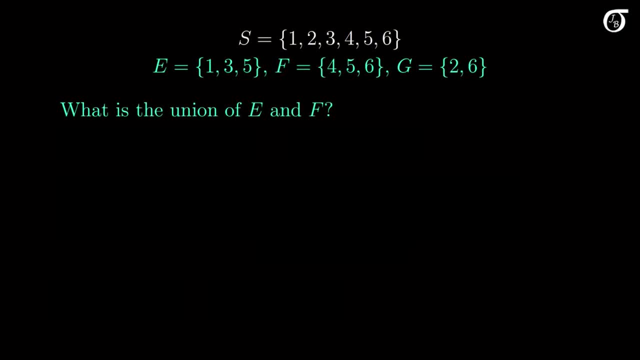 Now suppose we'd like to find the union of events E and F. The union of events E and F is 1 out of 6.. E and F is the set of sample points that are in either E or F or both. 1, 3, and 5 are in E, and 4,, 5, and 6 are in F. 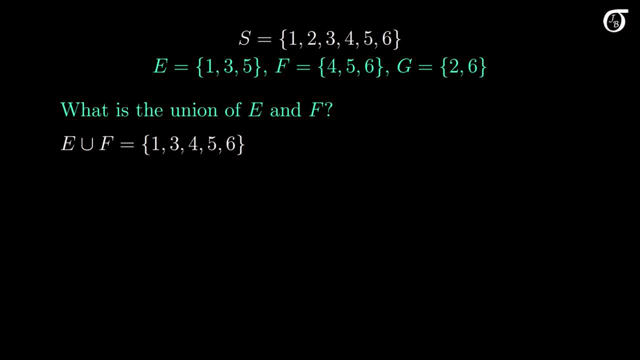 so E union F is made up of the numbers 1,, 3,, 4,, 5, and 6.. E union F is made up of 5 of the 6 equally likely sample points. so the probability of that union is 5 out of 6.. 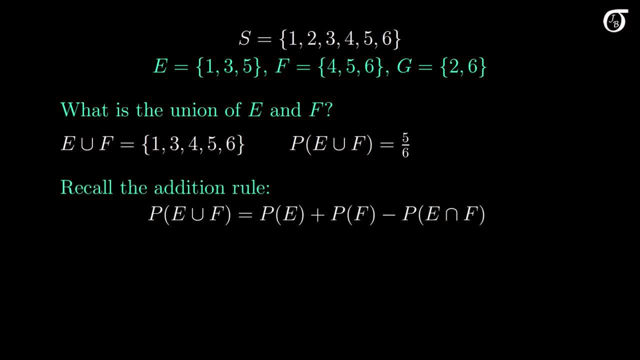 Alternatively to find the probability of their union, we could have used the addition rule. The probability of the union of E and F is the sum of the individual probabilities minus the probability of the intersection. E and F each have a probability of occurring of 3 out of 6,. 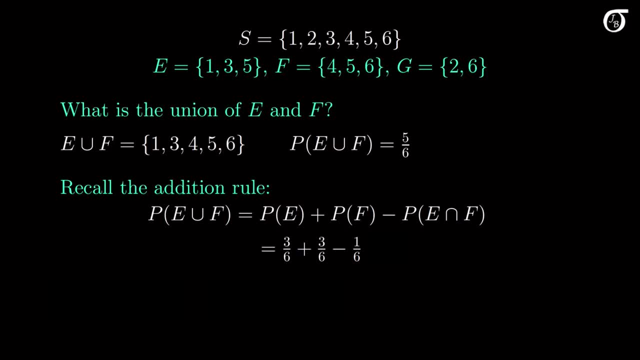 and we found in the previous slide that their intersection has a probability of 1 out of 6.. So by the addition rule, the probability of their union is 5 out of 6.. This is, of course, the same as what we found above using arguments based on the sample space. 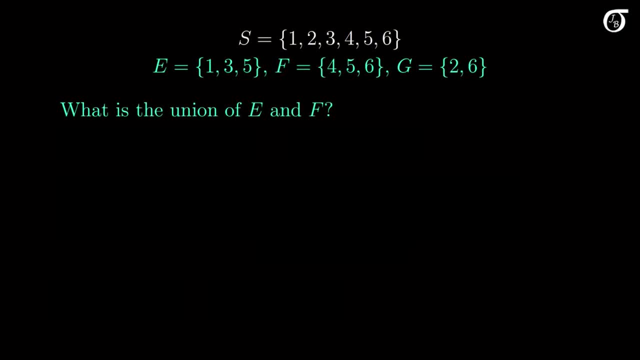 Now suppose we'd like to find the union of events E and F. The union of events E and F is 1 out of 6.. E and F is the set of sample points that are in either E or F or both. 1, 3, and 5 are in E, and 4,, 5, and 6 are in F. 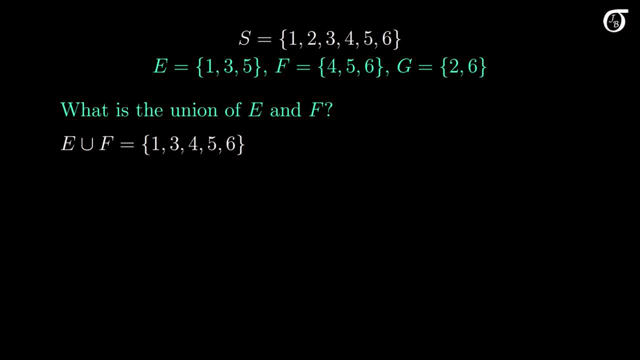 so E union F is made up of the numbers 1,, 3,, 4,, 5, and 6.. E union F is made up of 5 of the 6 equally likely sample points. so the probability of that union is 5 out of 6.. 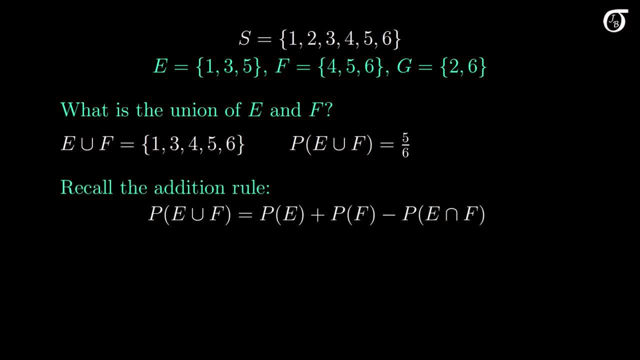 Alternatively to find the probability of their union, we could have used the addition rule. The probability of the union of E and F is the sum of the individual probabilities minus the probability of the intersection. E and F each have a probability of occurring of 3 out of 6,. 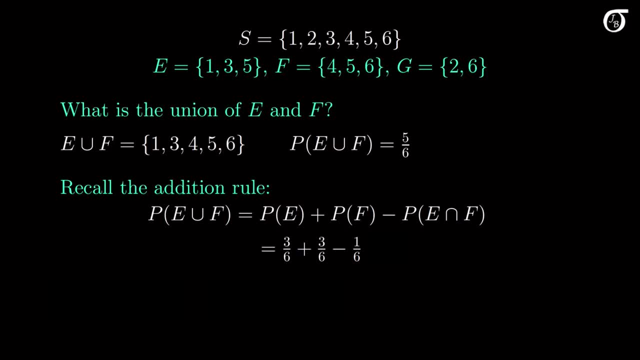 and we found in the previous slide that their intersection has a probability of 1 out of 6.. So by the addition rule, the probability of their union is 5 out of 6.. This is, of course, the same as what we found above using arguments based on the sample space. 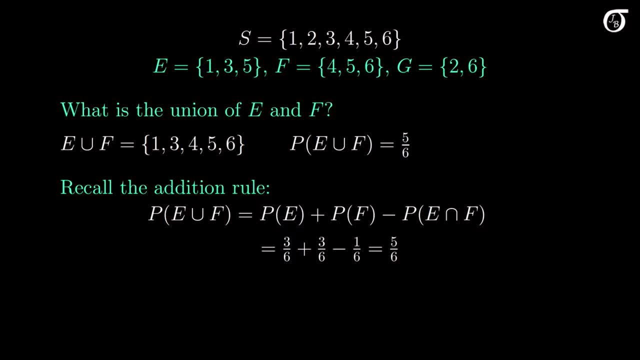 and our knowledge of what a union is. And if, say, we were interested in the complement of E, union F, that would simply be the number 2, as that is the only point in the sample space that is not in E or F. 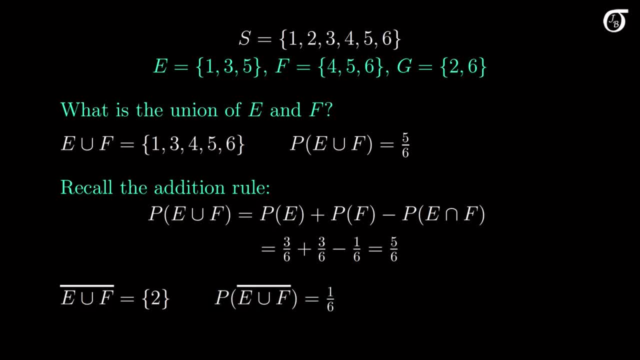 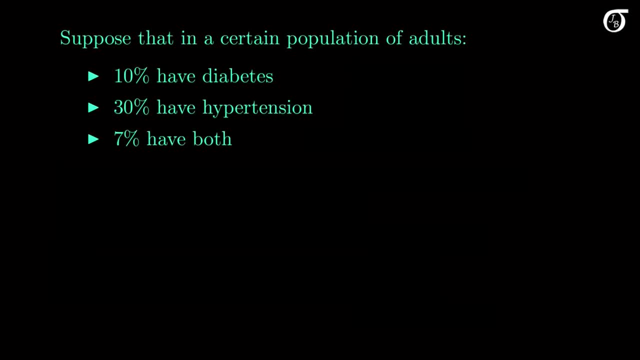 The probability of that complement is 1 out of 6.. Suppose that in a certain population of adults, 10% of diabetes, 30% of high blood pressure or, a little more formally, hypertension, and 7% have both. 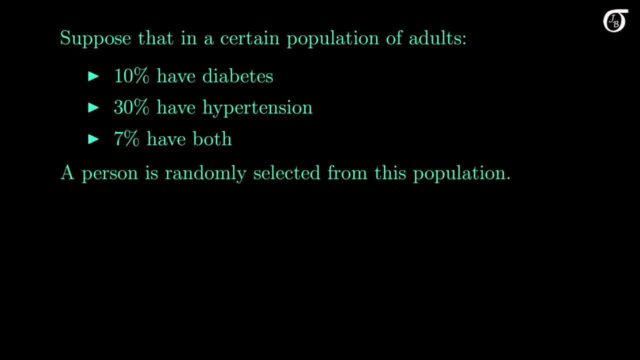 And suppose that a person is randomly selected from this population. Let event D represent the event that the randomly selected person has diabetes and event H represent the event that the person has hypertension. If we are randomly selecting from this population, then the probability the randomly selected person has diabetes is 0.1,. 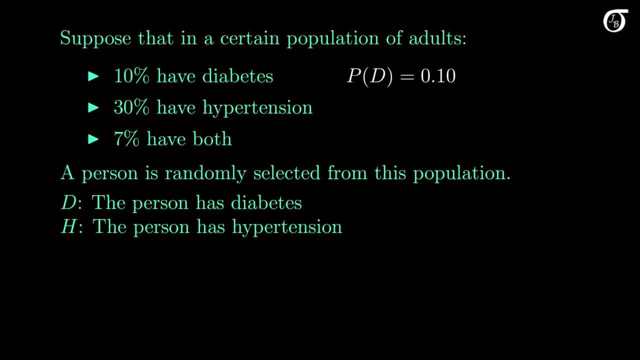 since 10% of the population has diabetes, The probability they have hypertension is 0.3, and the probability they have both is 0.07.. The complement of event D is the event the person does not have diabetes by the complement rule. 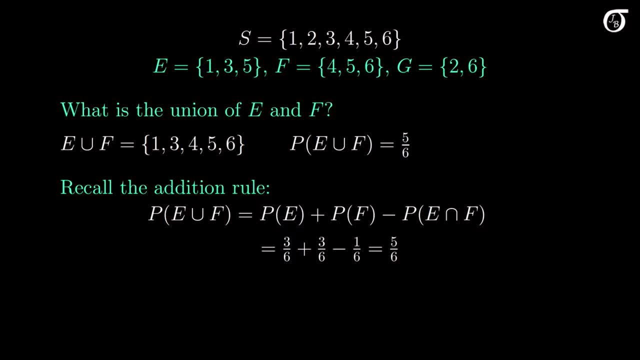 and our knowledge of what a union is. And if, say, we were interested in the complement of E, union F, that would simply be the number 2, as that is the only point in the sample space that is not in E or F. 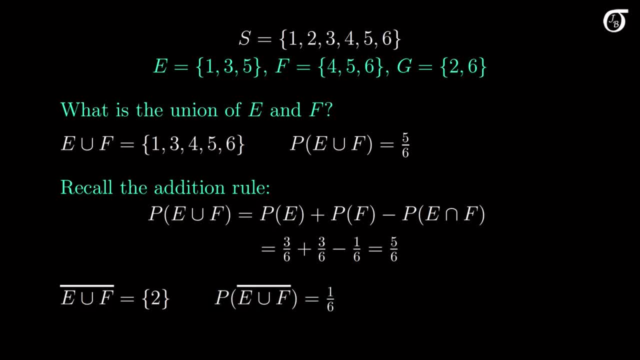 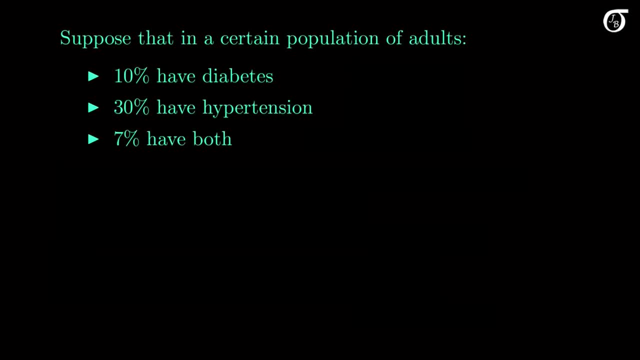 The probability of that complement is 1 out of 6.. Suppose that in a certain population of adults, 10% of diabetes, 30% of high blood pressure or, a little more formally, hypertension, and 7% have both. 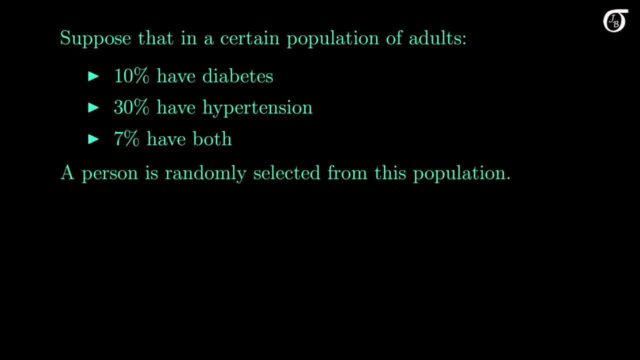 And suppose that a person is randomly selected from this population. Let event D represent the event that the randomly selected person has diabetes and event H represent the event that the person has hypertension. If we are randomly selecting from this population, then the probability the randomly selected person has diabetes is 0.1,. 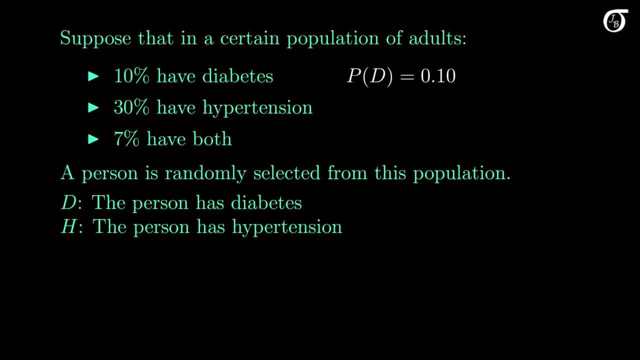 since 10% of the population has diabetes, The probability they have hypertension is 0.3, and the probability they have both is 0.07.. The complement of event D is the event the person does not have diabetes by the complement rule. 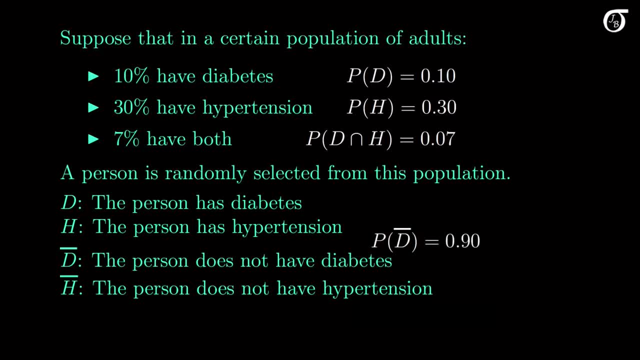 the probability the person does not have diabetes is 1-0.1, or 0.9.. The complement of event H is the event the person does not have hypertension. By the complement rule, the probability the person does not have hypertension is 1-0.3, or 0.7.. 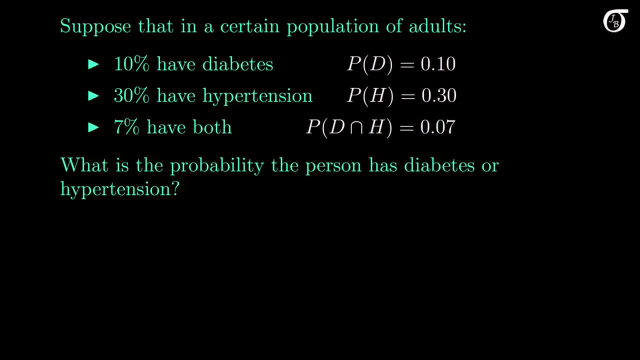 Now suppose we want to know the probability the person has diabetes or hypertension or both. That's the probability of the union of events D and H. And we can find that with the addition rule The probability of D union H is the probability of D plus the probability of H. 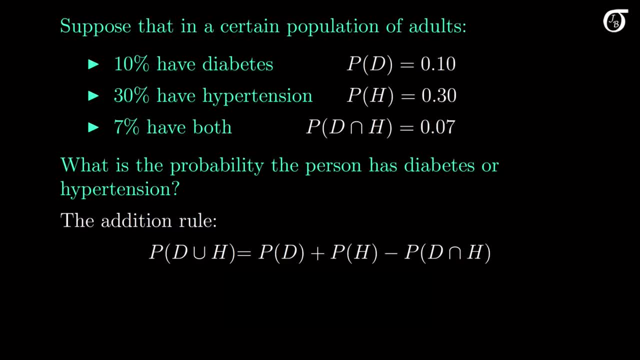 minus the probability of the intersection of D and H. All three of those probabilities are given here and in the end we find the probability that the person has diabetes or hypertension is 0.33.. And again, that's, or in the inclusive sense. 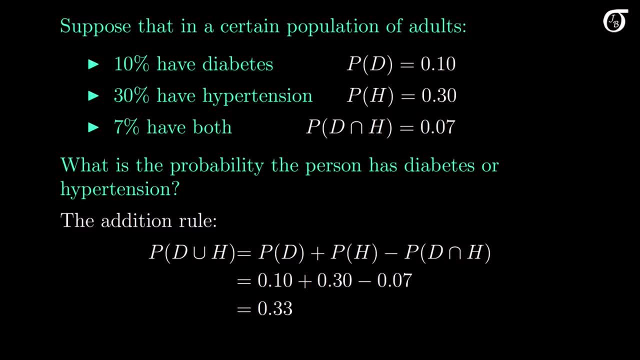 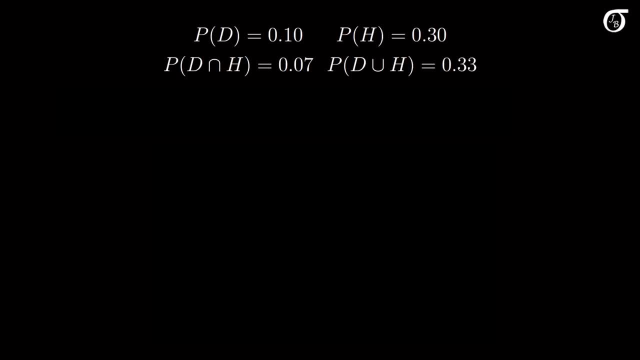 the probability they have diabetes or hypertension or both. It's often helpful to illustrate the events and the probabilities that relate to them in a Venn diagram. Let's look at how we might do that here. Here are the four probabilities that we've been given or we've worked out so far. 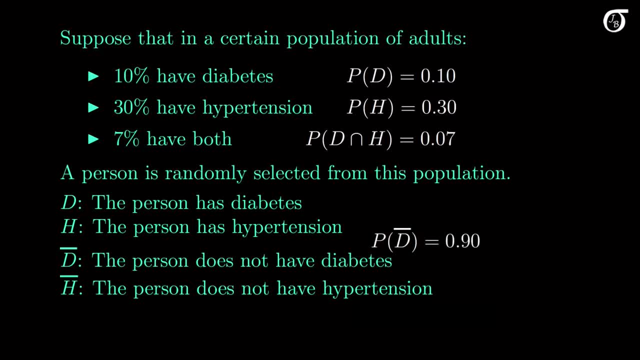 the probability the person does not have diabetes is 1-0.1, or 0.9.. The complement of event H is the event the person does not have hypertension. By the complement rule, the probability the person does not have hypertension is 1-0.3, or 0.7.. 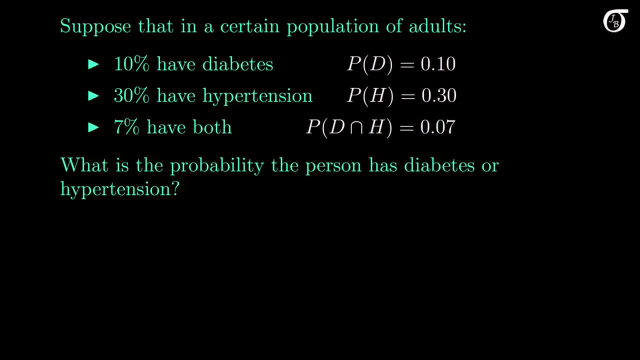 Now suppose we want to know the probability the person has diabetes or hypertension or both. That's the probability of the union of events D and H. And we can find that with the addition rule The probability of D union H is the probability of D plus the probability of H. 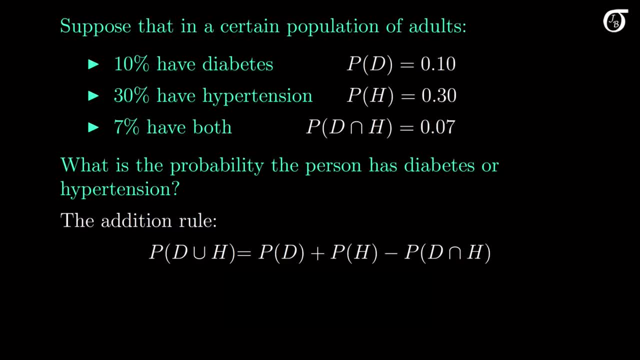 minus the probability of the intersection of D and H. All three of those probabilities are given here and in the end we find the probability that the person has diabetes or hypertension is 0.33.. And again, that's, or in the inclusive sense. 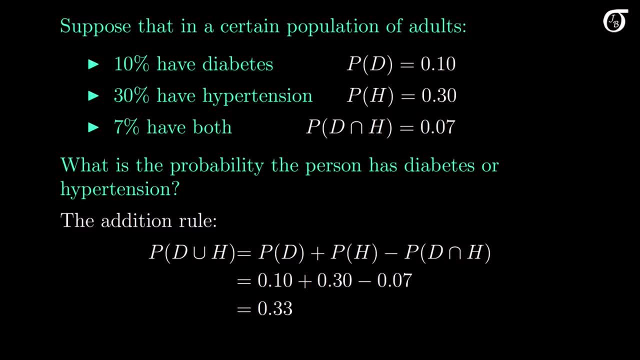 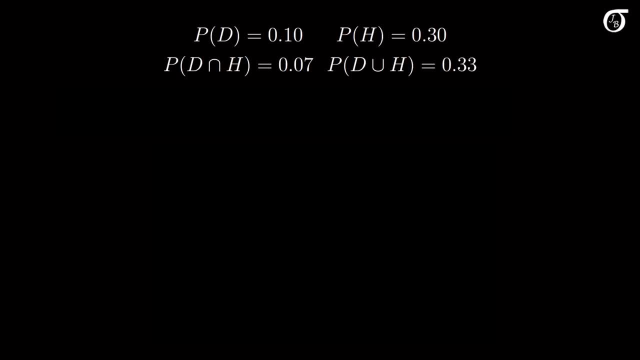 the probability they have diabetes or hypertension or both. It's often helpful to illustrate the events and the probabilities that relate to them in a Venn diagram. Let's look at how we might do that here. Here are the four probabilities that we've been given or we've worked out so far. 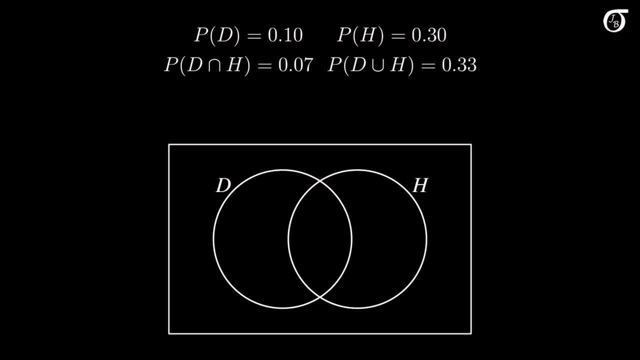 And here's a Venn diagram illustrating events D and H. In a typical Venn diagram, like the one we're using here, the sizes of the various regions, such as the size of circle H, don't have any meaning. The Venn diagram simply illustrates the various regions. 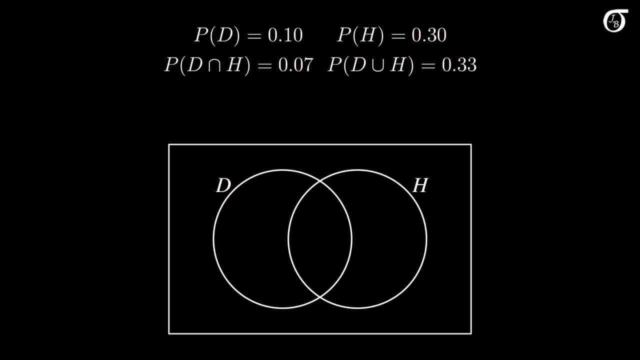 So try not to read into the size of the regions in a typical Venn diagram. Now let's fill in the various regions and their probabilities of occurring. The event the person has both diabetes and hypertension is represented by D, intersect H, and that's this green region. 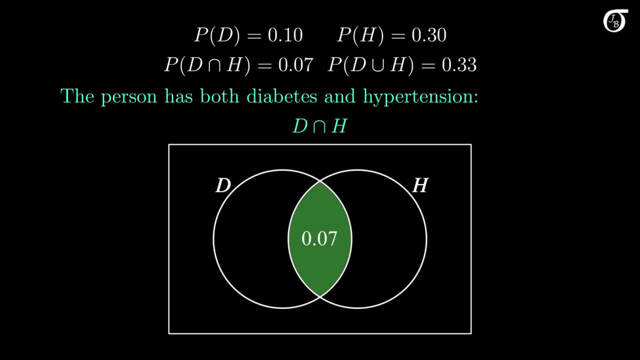 That probability was given to us as 0.07, so I'm going to put that value in here. The event that the person has diabetes but not hypertension is represented by D, intersect H complement, and that's this green region. Since the entire event D has a probability of occurring of 0.1,. 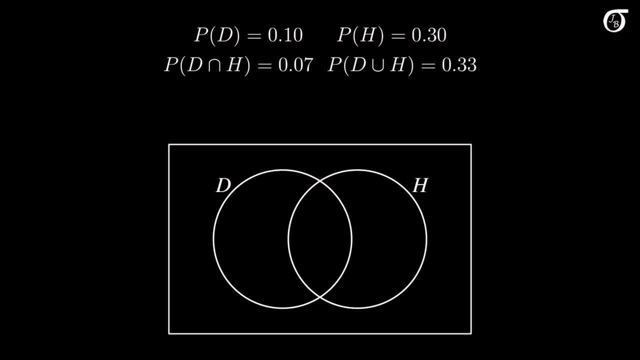 And here's a Venn diagram illustrating events D and H. In a typical Venn diagram, like the one we're using here, the sizes of the various regions, such as the size of circle H, don't have any meaning. The Venn diagram simply illustrates the various regions. 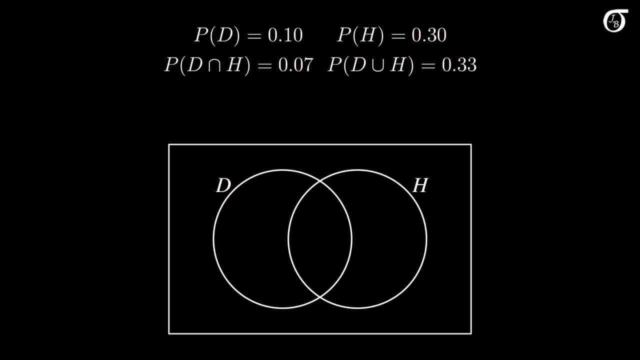 So try not to read into the size of the regions in a typical Venn diagram. Now let's fill in the various regions and their probabilities of occurring. The event the person has both diabetes and hypertension is represented by D, intersect H, and that's this green region. 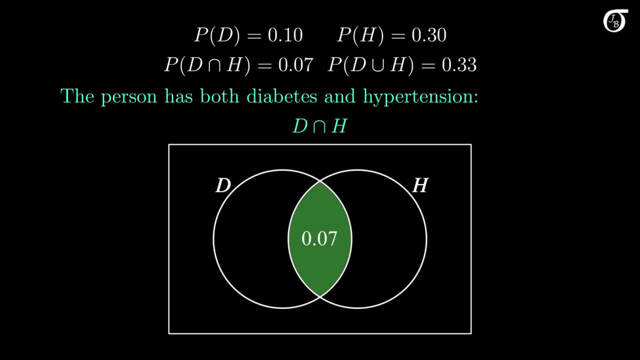 That probability was given to us as 0.07, so I'm going to put that value in here. The event that the person has diabetes but not hypertension is represented by D, intersect H complement, and that's this green region. Since the entire event D has a probability of occurring of 0.1,. 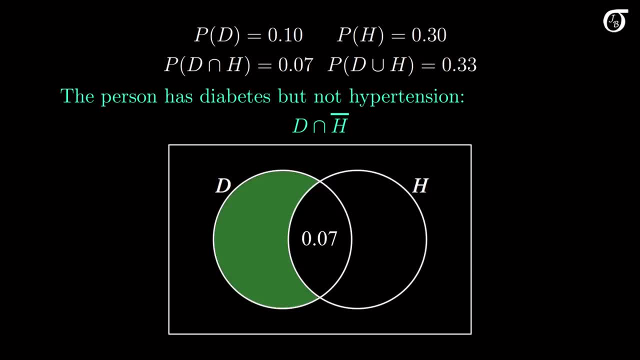 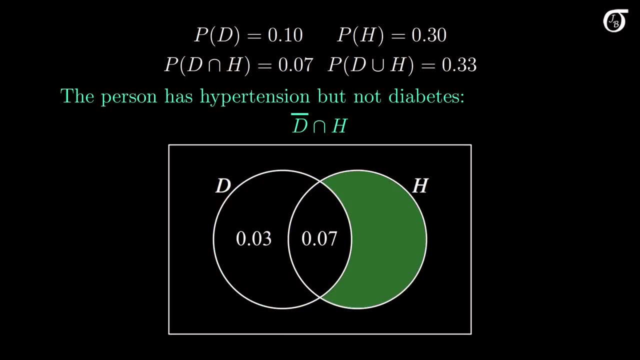 the probability associated with this green region representing diabetes but not hypertension must be 0.03.. The event that the person has hypertension but not diabetes can be represented by D complement intersect H, Or I could flip those two around if I wanted to. 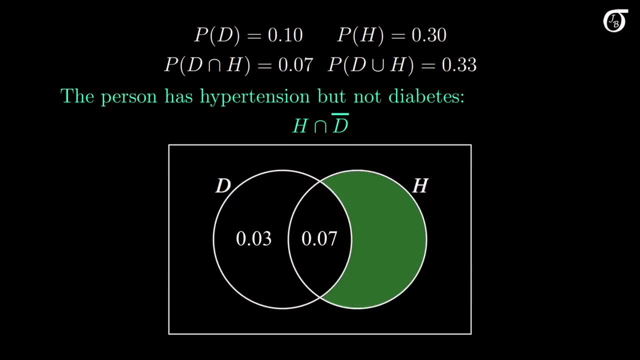 to be more consistent with the wording, as the ordering of events in an intersection doesn't matter, And that's this region in green. The probability of H in its entirety is 0.3, so the probability of this green region alone must be 0.23. 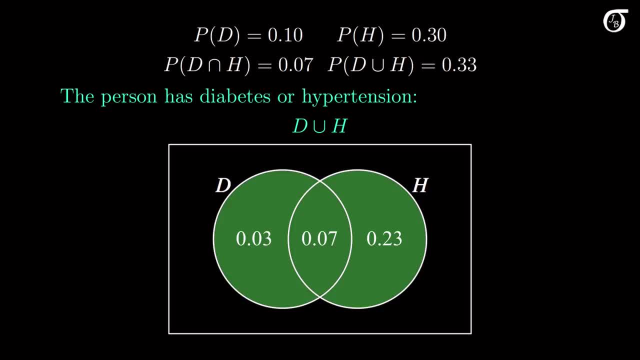 The event that the person has diabetes or hypertension is the union of D and H, represented by this green region. We've already found the probability of the union of those events to be 0.33 using the addition rule, but we could also find it here by adding up the three probabilities. 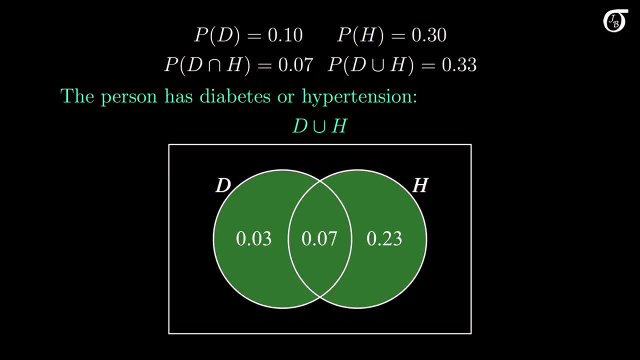 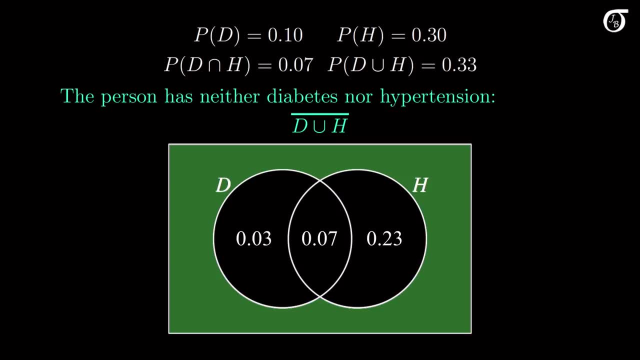 of the three mutually exclusive regions that we see here. 0.03 plus 0.07 plus 0.23 is 0.33.. How about the event that the person has neither diabetes nor hypertension? One way of writing, that is, by recognizing that this event is the complement of the union. 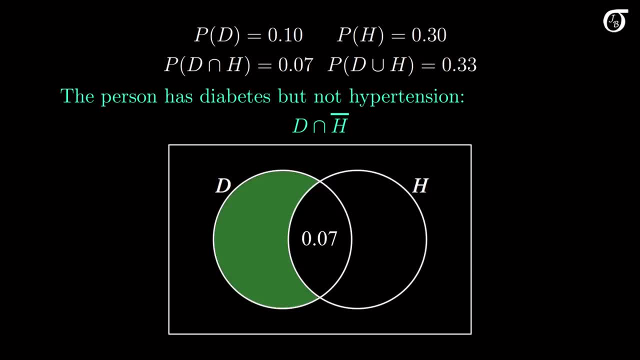 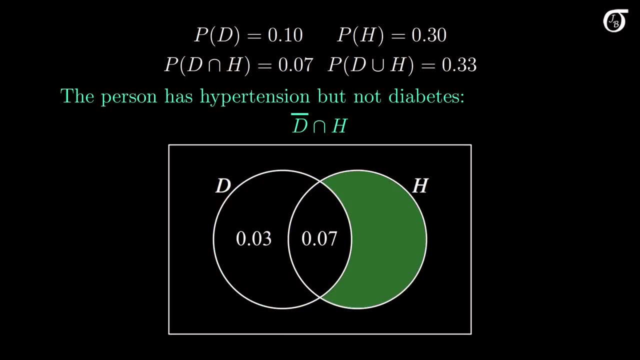 the probability associated with this green region representing diabetes but not hypertension must be 0.03.. The event that the person has hypertension but not diabetes can be represented by D complement intersect H, Or I could flip those two around if I wanted to. 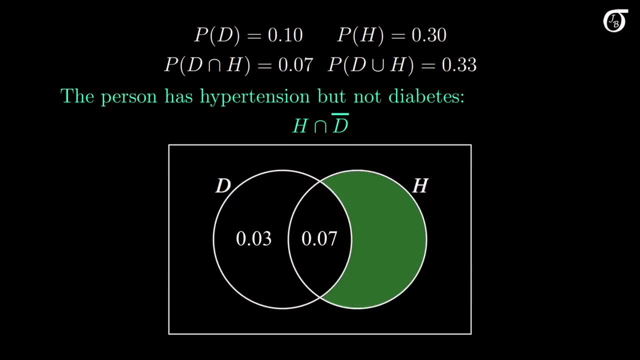 to be more consistent with the wording, as the ordering of events in an intersection doesn't matter, And that's this region in green. The probability of H in its entirety is 0.3, so the probability of this green region alone must be 0.23. 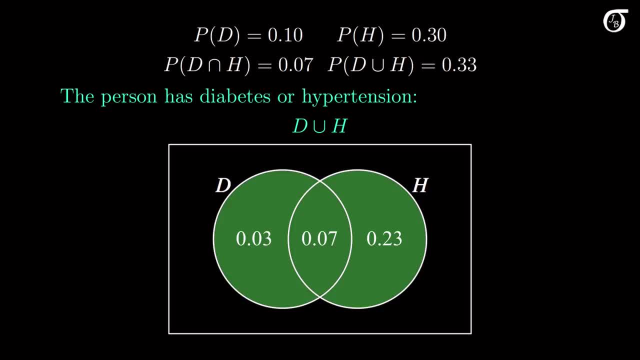 The event that the person has diabetes or hypertension is the union of D and H, represented by this green region. We've already found the probability of the union of those events to be 0.33 using the addition rule, but we could also find it here by adding up the three probabilities. 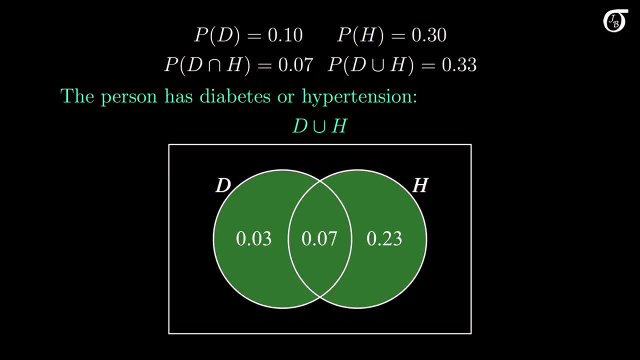 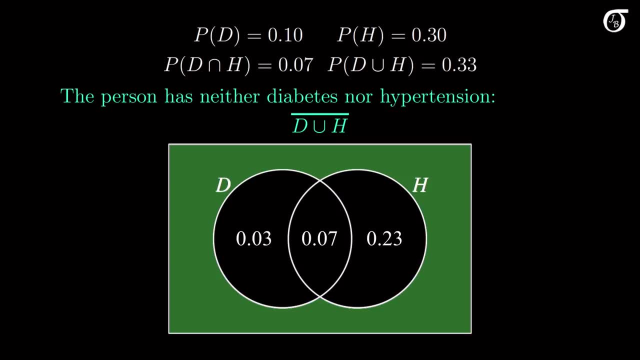 of the three mutually exclusive regions that we see here. 0.03 plus 0.07 plus 0.23 is 0.33.. How about the event that the person has neither diabetes nor hypertension? One way of writing, that is, by recognizing that this event is the complement of the union. 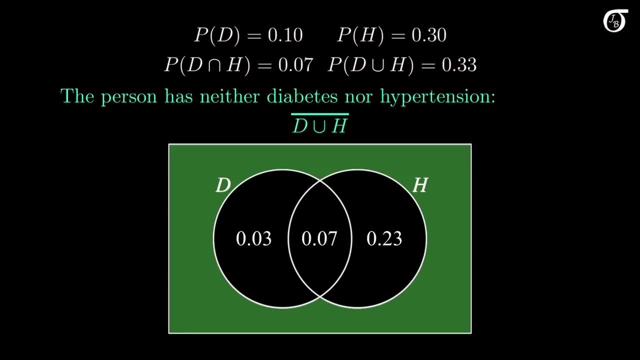 The union is that they have either one or the other. So the complement of the union is that they have neither. That's this green region, And since the probability of the entire sample space is 1, the probability associated with this event must be 0.67.. 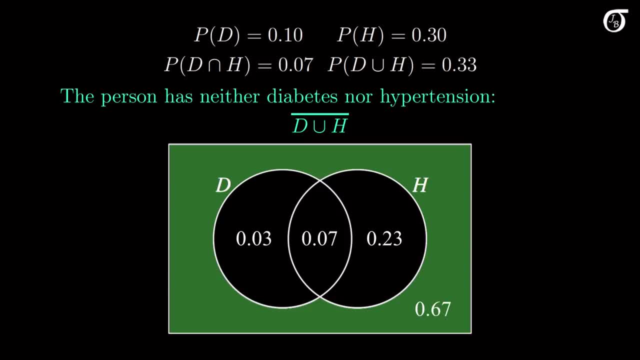 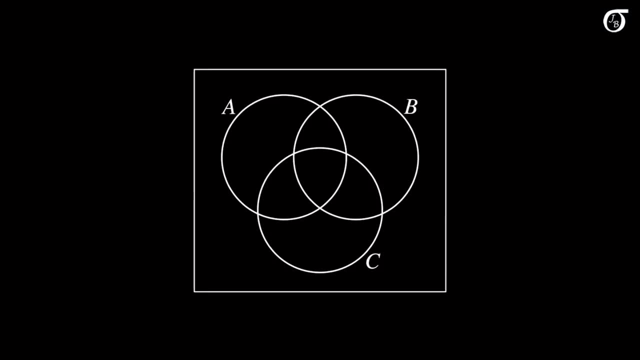 Setting up a Venn diagram like this often helps us visualize probability problems and makes them much easier to solve. The concepts of unions, intersections and complements can be extended to more than two events. For example, here's a Venn diagram representing three events: A, B and C. 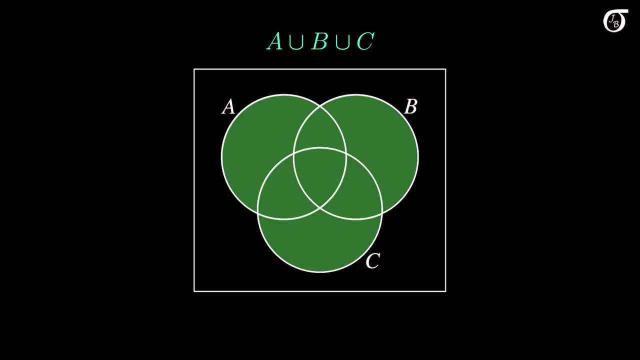 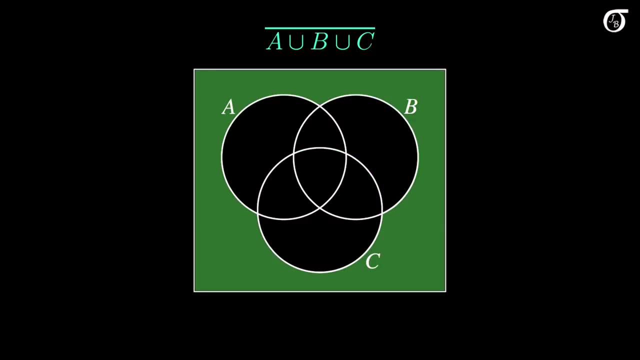 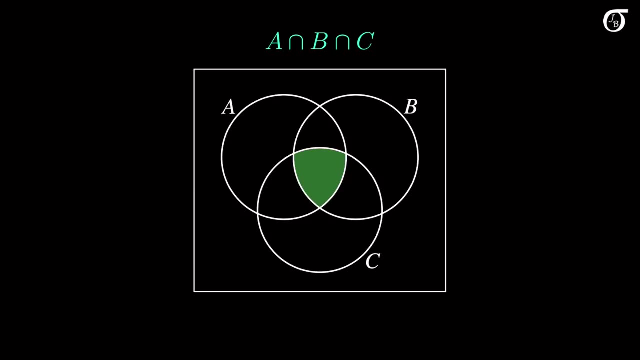 The union of events A, B and C is this green region where A or B or C occurs. The complement of that union is this green region where neither A nor B nor C occurs. The intersection of A, B and C is the event that A and B and C occur.